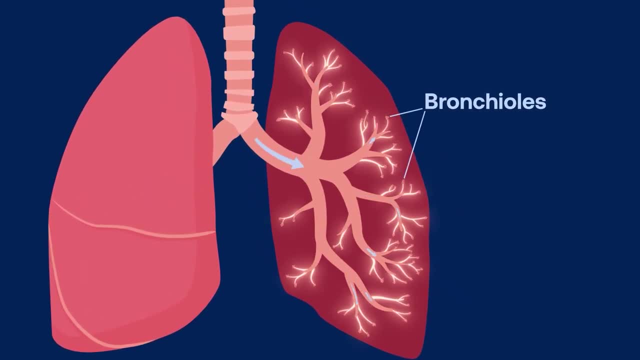 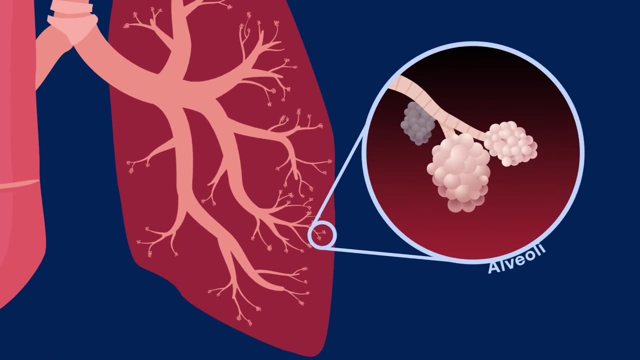 then separate into small tubes called bronchioles. Like tree branches, bronchioles divide into thousands of even smaller passages. At the end of each bronchiole is a cluster of little air sacs called alveoli. Alveoli are wrapped in tiny blood vessels called capillaries. 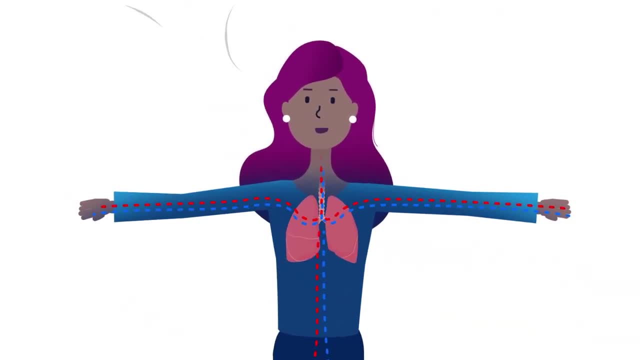 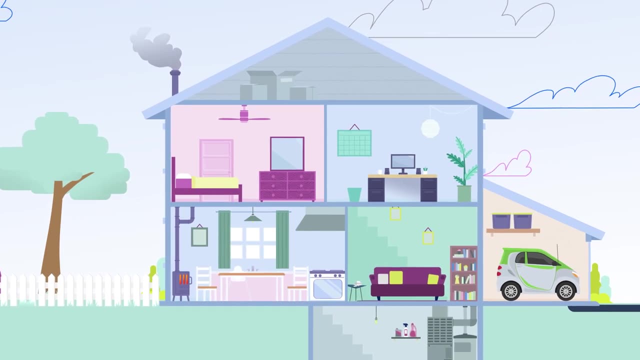 The air you breathe in fills these air sacs with oxygen-rich air. Here is where oxygen is transported throughout the body. Not all the air you breathe in is clean. Indoor air contaminants can include small particles that are suspended in the air. When those particles 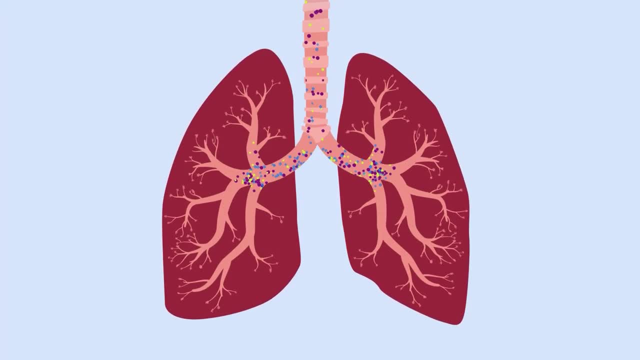 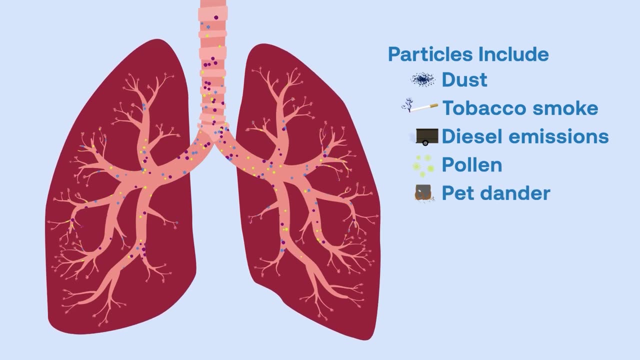 from the air travel deep into your body. they can have a negative impact on your body. These particles can include things like dust, tobacco smoke, diesel emissions, pollen, pet dander, mold spores, chemicals, gases and more Particulate matter often written. 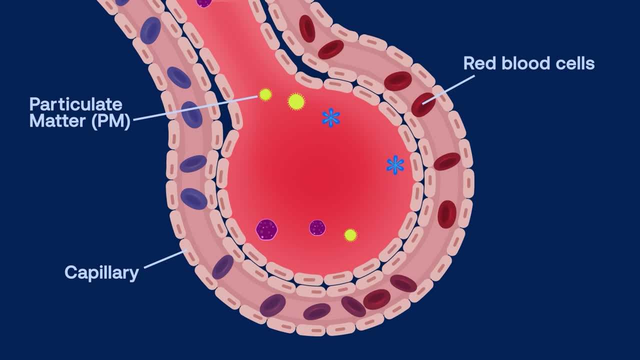 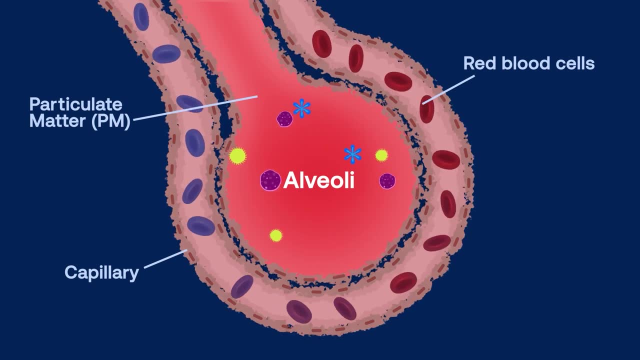 as PM are so small, they go into the lungs all the way to the alveoli. Once there, they can irritate and corrode the alveoli wall, damaging the lungs and causing lung disease. Healthier in schools can benefit: students, teachers and others. 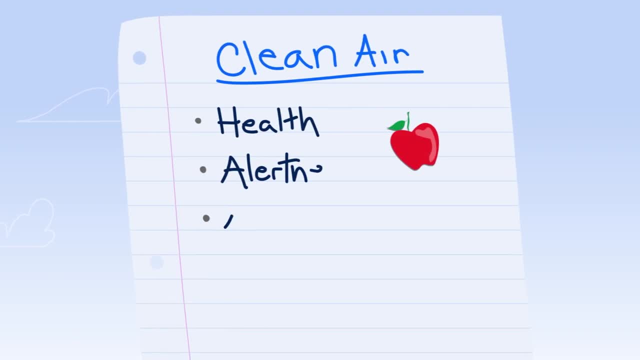 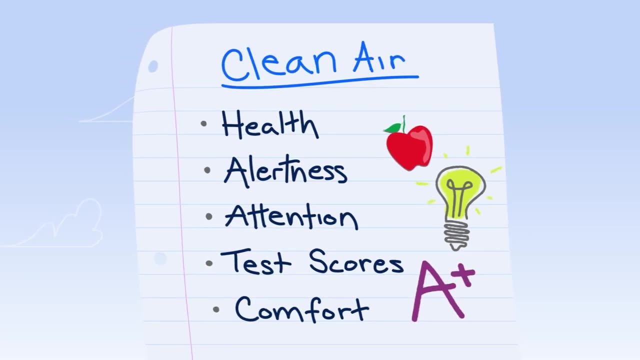 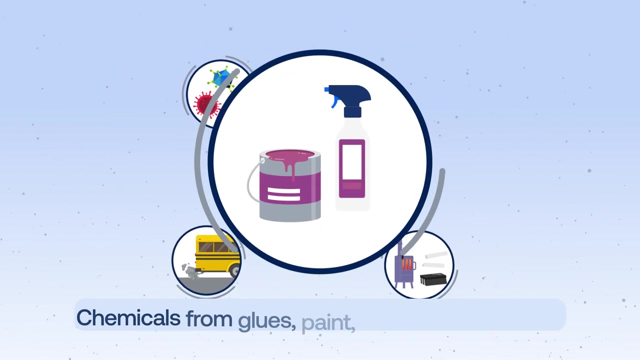 Clean air can improve health, alertness, attention, test scores and comfort for both students and teachers. But not all the air we breathe in school is clean. School air may have several pollutants, including mold, bacteria and viruses, chemicals from glues. 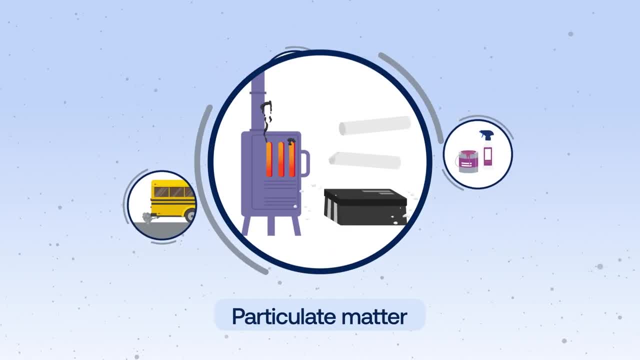 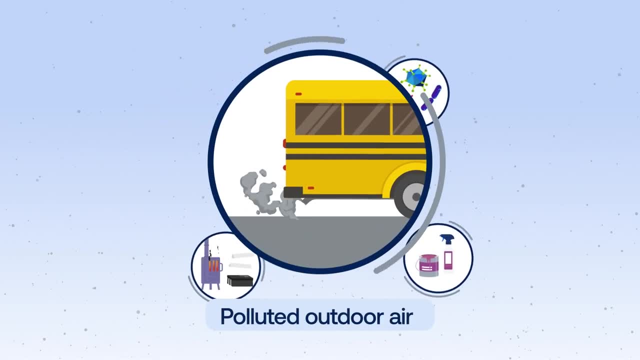 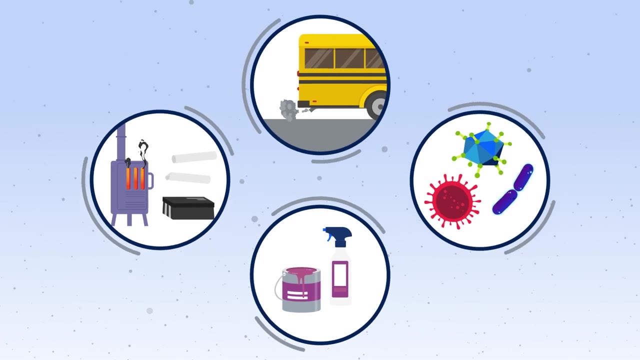 paint or cleaning supplies, particulate matter from chalk, dust, soil, new furniture, cooking carpets, heaters and wood stoves. Also polluted outdoor air from busy traffic, nearby factories and wildfires can come inside the school. To improve the indoor air quality in your school, remove the source of the air pollution. 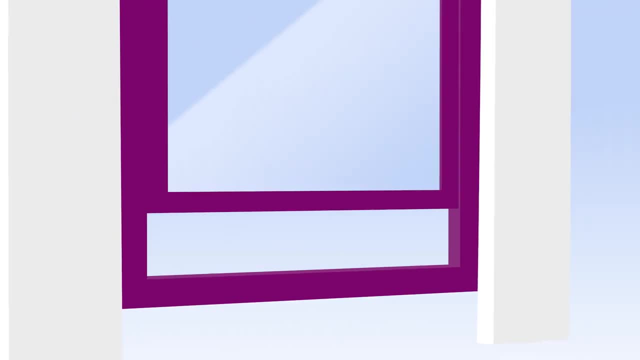 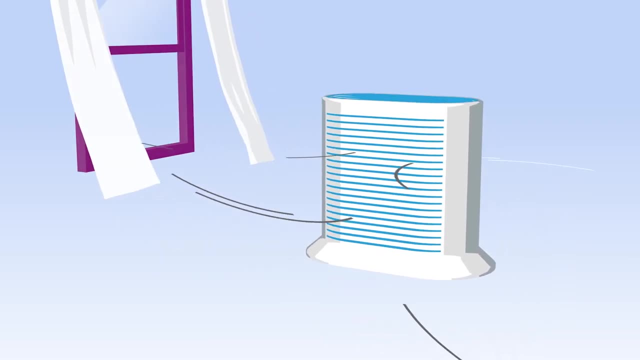 if you can. Prevention is best. Air out your classroom by opening doors and windows. Filter the air with an air cleaner. Air cleaners take in the room's air and capture particles, viruses and many chemicals. The air cleaners then release clean air back into the room. 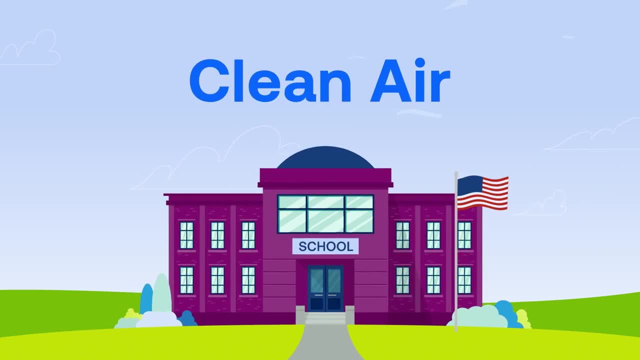 Learning how to protect yourself from poor air quality doesn't have to be hard. Visit longedu org to learn more.